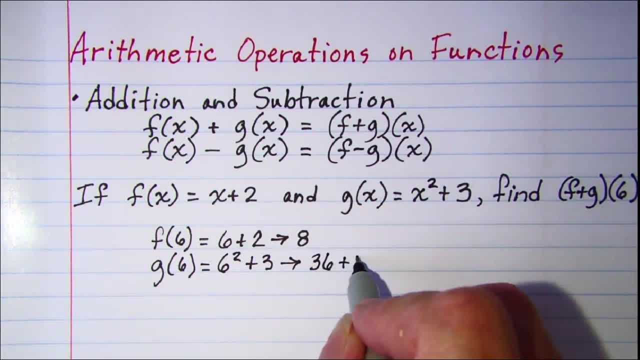 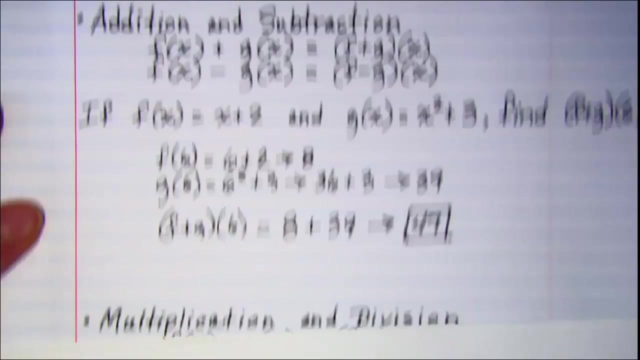 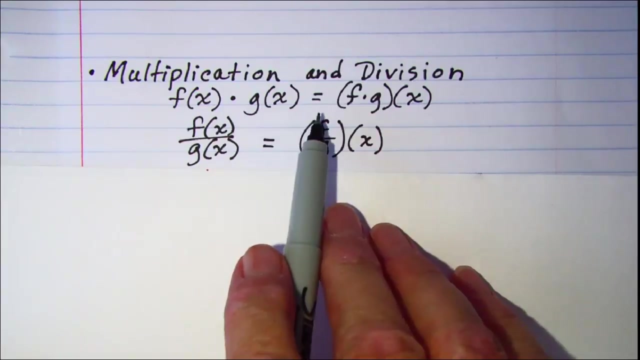 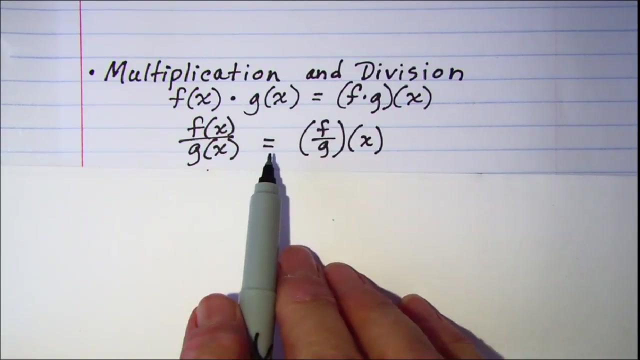 is 36 plus 3 is 39. So then f plus g of 6 will equal f of 6 plus g of 6 or 47.. During multiplication and division: For multiplication and division: For multiplication and division, f times g of x and f of x divided by g of x is equal to f divided by g of x. 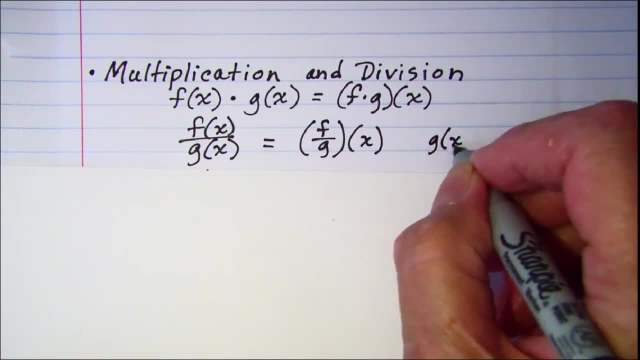 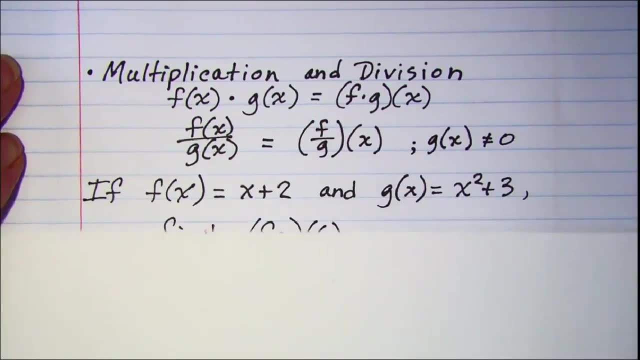 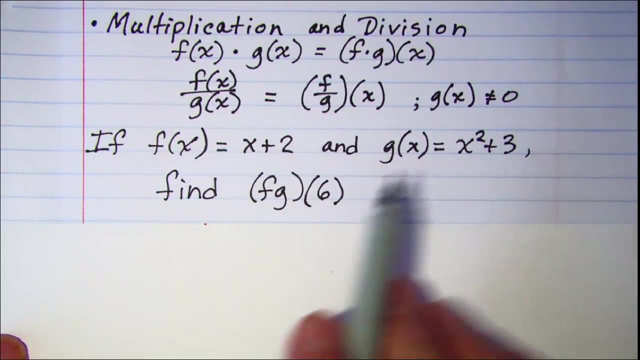 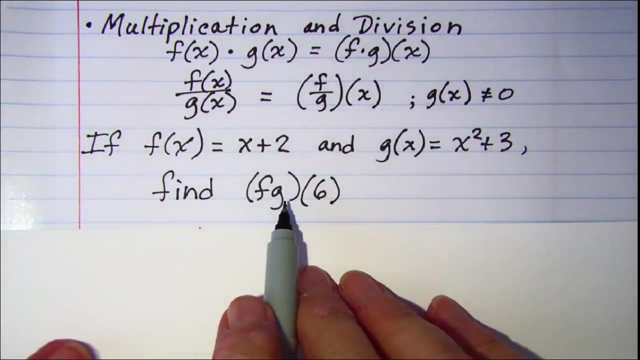 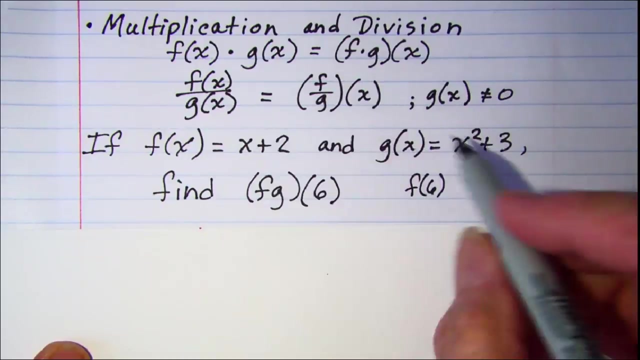 Remember that our denominator cannot equal zero, so g of x cannot equal zero. If f of x is equal to x plus 2 and g of x is equal to x squared plus 3, find f times g of 6.. So again we can find f of 6 by substituting 6 into the f function. 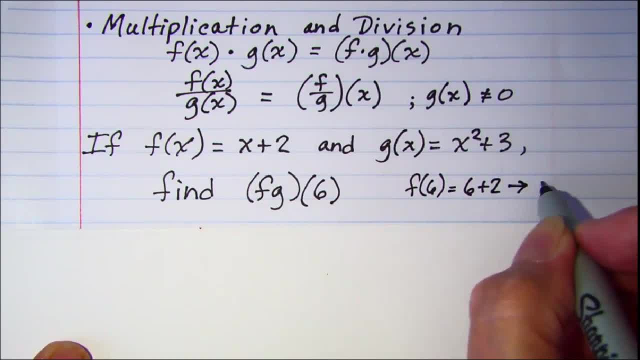 That's going to be 6 plus 2 or 8. We can find g of 6. by substituting 6. 6 into the g function. so that's 6 squared plus 3 is 36 plus 3 is 39, and so 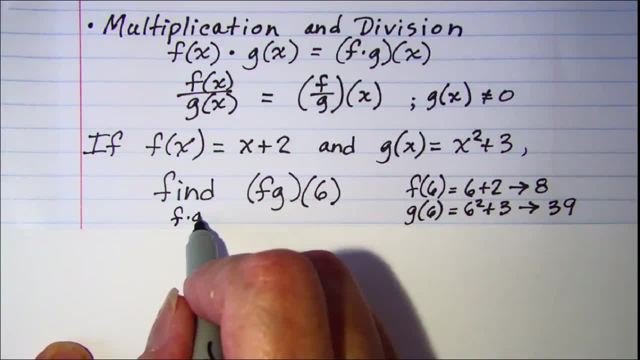 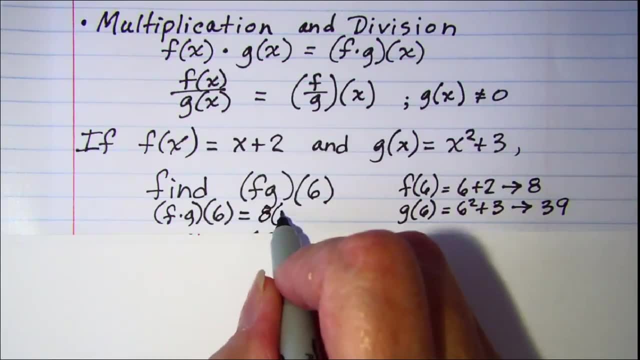 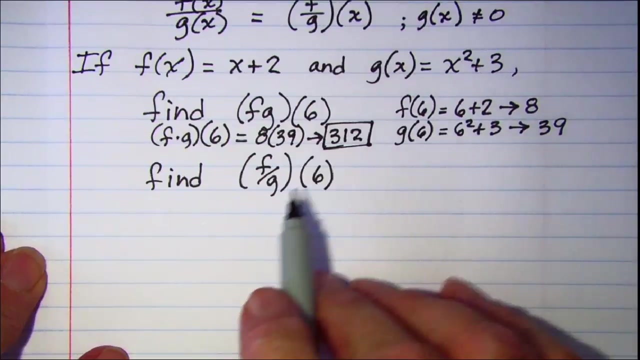 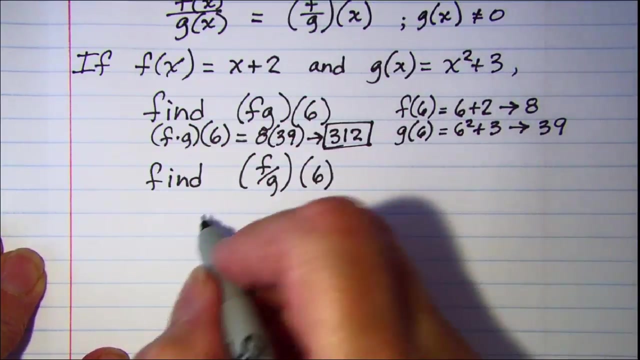 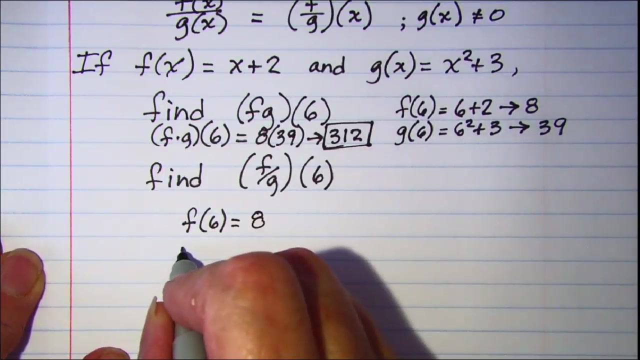 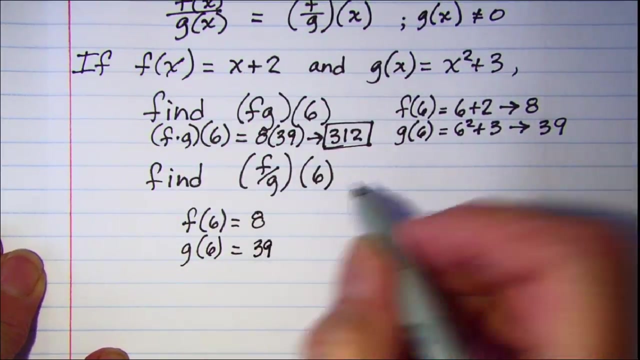 then we have f times g of 6 will equal 8 times 39, or 312 for f divided by g of 6. again we've got found f of 6, we know that f of 6 is 8, and we know that g of 6 is 39. so 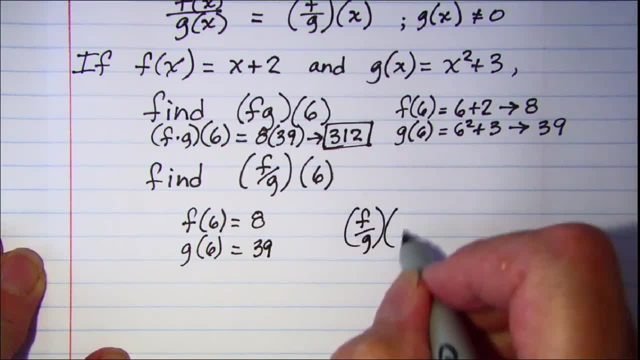 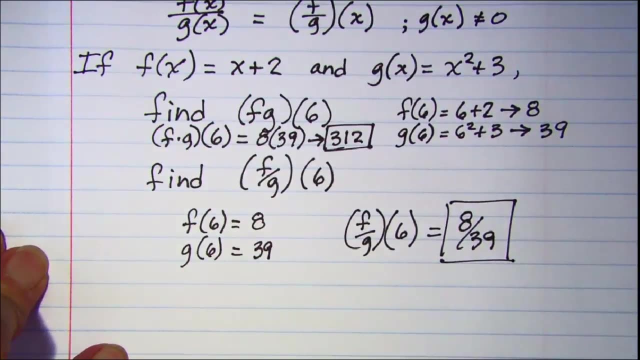 f divided by g of 6 will equal 8 over 39. now, this fraction cannot be simplified any. so that is our product.